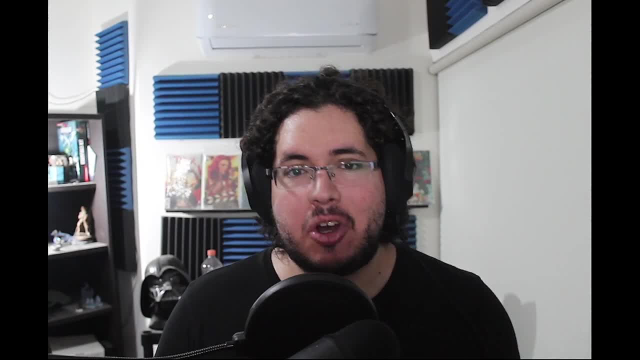 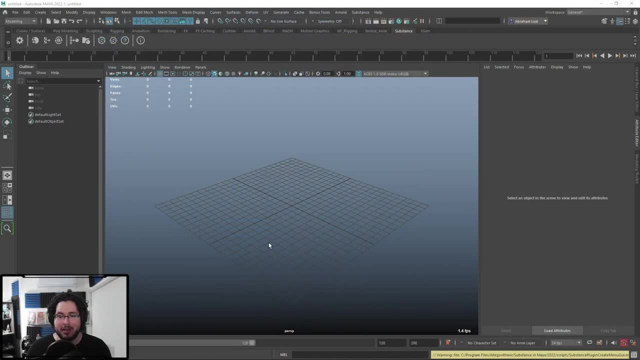 Hey guys, welcome to the next video in this channel. So what's the deal, right? Why am I wearing a black shirt today? Well, let me tell you a little story while I open. Maya, So I was preparing laundry today and we were doing our laundry and the weather here changed like. erratically. It was really, really sunny. That's why we were doing laundry, because we wanted to place the cloths outside for them to dry And suddenly we had like a thunderstorm and then super heavy rain and hail and everything. So it was crazy. It was crazy. So, unfortunately, 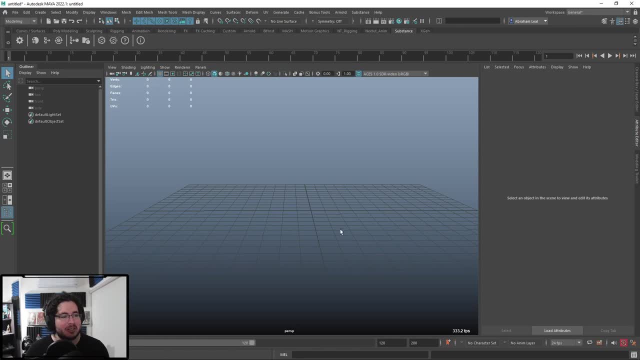 I don't have my uniform right now. I don't have my Nextud branding shirt, So I apologize. This is going to be the only video, probably, that you're going to see me with like a non-Nextud shirt, But yeah, so let's get to it. As I mentioned, I'm still in the process of recording the Marmoset. 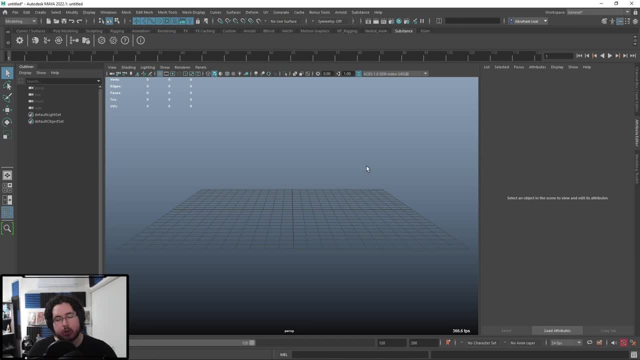 videos. So this next couple of videos, which is going to be the one that I'm recording today and the ones from the next couple of days, are going to be some quick tips about topology. Topology is one of those things that I'm going to be talking about in the next couple of days, So I'm going to 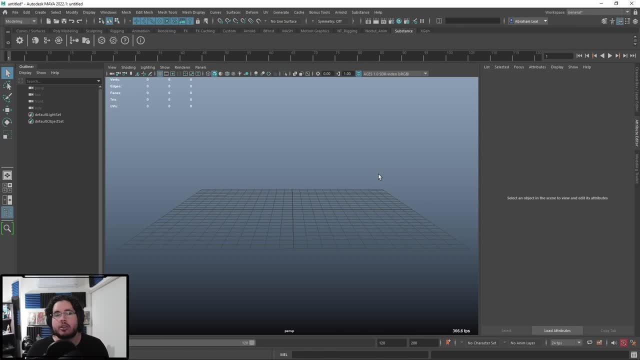 be talking about some of those topics. that's very mysterious at first. When you first start learning 3D, you don't really know why topology is important. So I want to show you some couple of nice little tips and tricks that are going to be helping you create some very nice geometries. 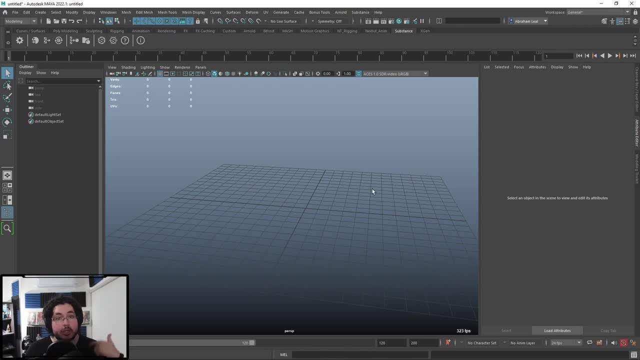 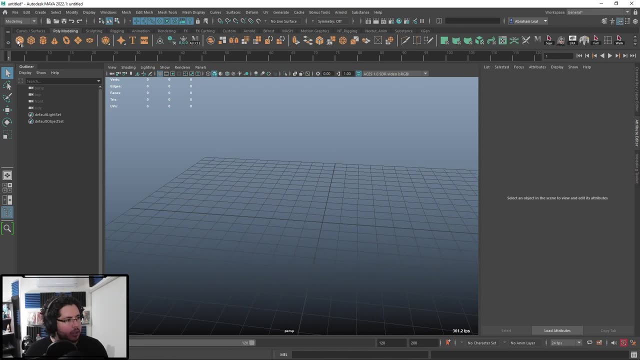 and models, And now this applies to anything. It could be for Maya, for Blender, for anything. So it's like a universal concept about 3D modeling. So what is topology? Well, topology is just the organization of your mesh, your squares and your triangles in any given model that you have, And 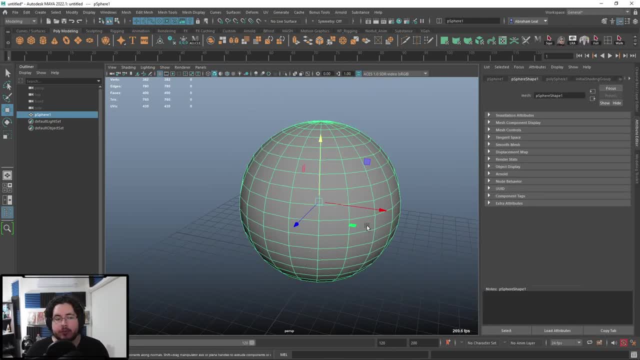 there's a couple of rules that we like to follow when we're doing topology. So, first of all, the rules that we like to follow in the 3D world. The first of them is we always use quads and triangles At render time, every single thing that you have is going to be triangulated, So even 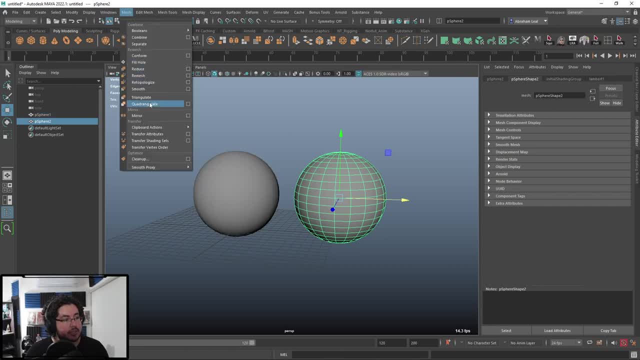 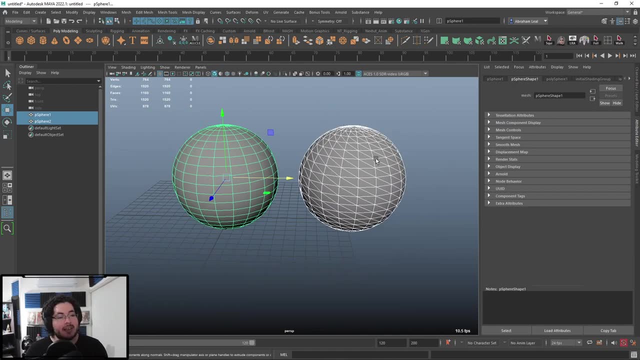 though we see this as quads, Maya, at render time, is going to see this as triangles. However, for our very- let's call it very- limited human mind, it's very difficult to see a shape like this and understand how things are like properly flowing. So that's why we like squares and boxes, because 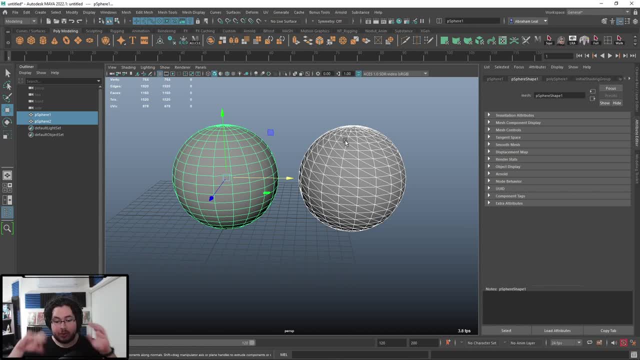 it's easier to think with like just those four shapes rather than thinking about like triangles all of a sudden. So that's why we like squares and boxes, because it's easier to think with like triangles all of a sudden. So the way in which you organize your quads and your triangles. 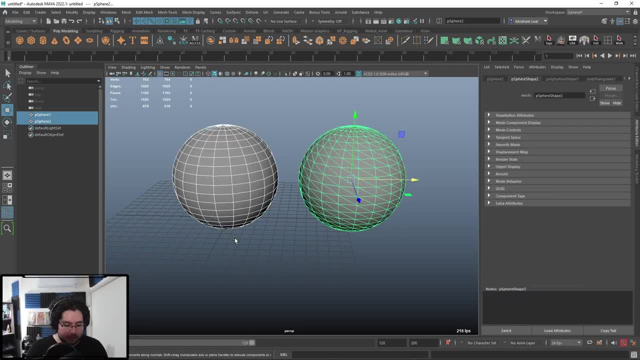 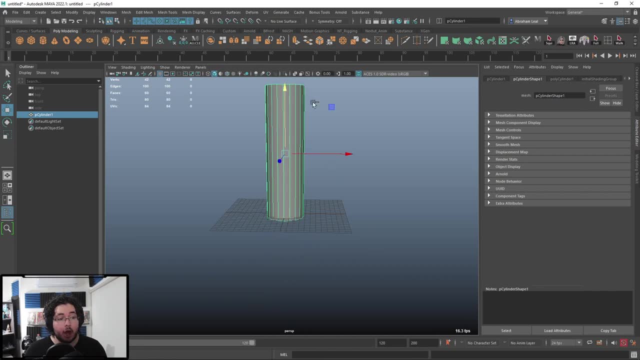 that's what we call topology. Now, why is topology important? Well, the main reason why topology is important is due to something called deformation, And that means that every now and then, you're going to have objects that are going to be deforming, especially when you're doing animated 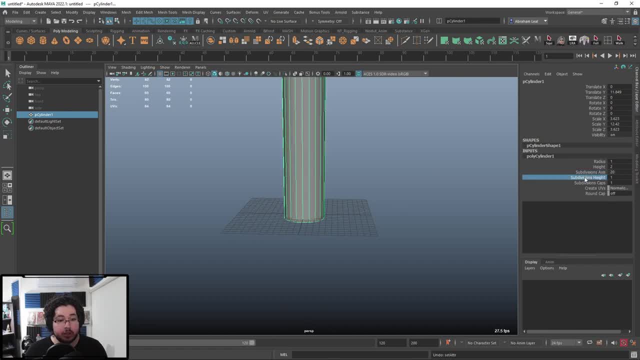 things. So topology, for instance, if you're doing 3D printing, which I'll show you in a second, you don't really need to worry about topology because you're not going to be deforming the object. But if you have this cylinder right here and you want to bend it, you're going to need 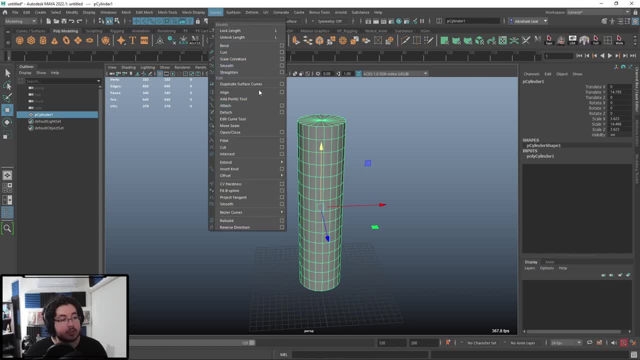 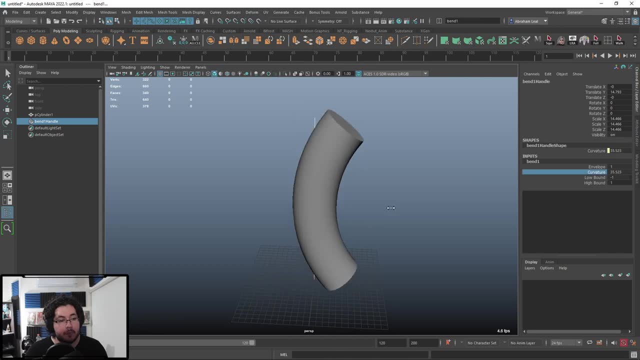 a proper subdivision of quads and triangles to make sure that the deformation that you apply to it- like here, let's say it's just like a nonlinear bend- it deforms nicely right, Like we create this very nice C shape. So that's why topology is important And I'm going to do the exact same. 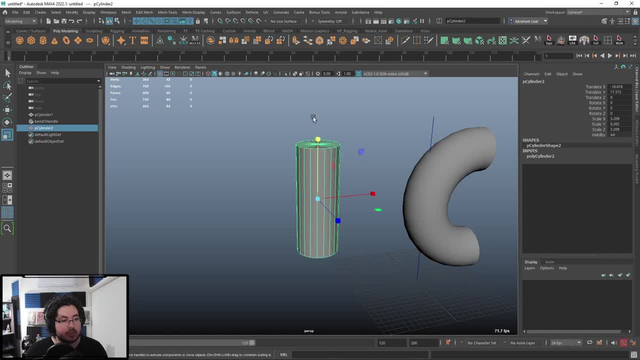 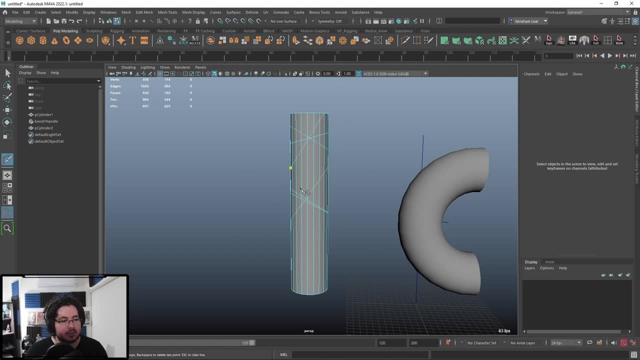 example. but now with like a bad topology. So let's say I have this triangle and I don't, or this triangle, this cylinder, and I don't care about topology, And I just start adding like angles and things like all around the place And I'm like, yeah, look at me, mom. 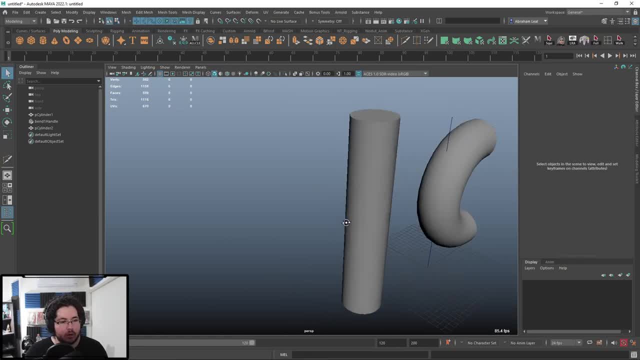 I'm 3D modeling. I'm super cool. It's like no one's going to know, right, Like you say this and you're like, yeah, that's a cylinder, All right. But then you see the topology and it's. 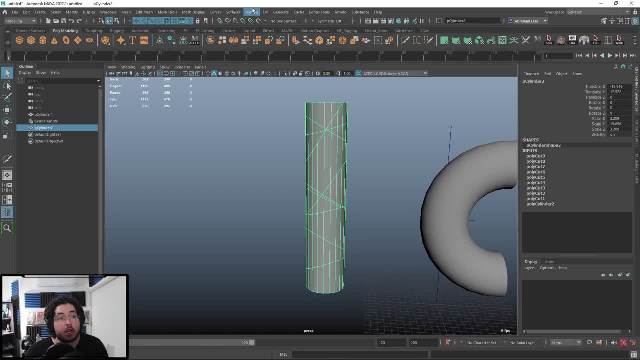 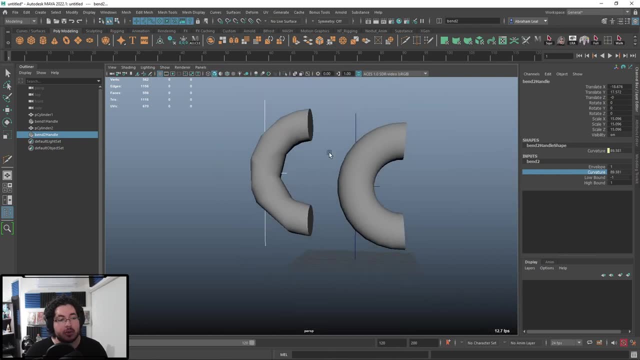 like: oh my God, that's horrible. And not only is it horrible, it's not going to deform properly. So if we go here into the form and bend and do the exact same thing, you're going to see that the deformation is not going to be. it's nowhere near clean as what we have right here. Okay, So 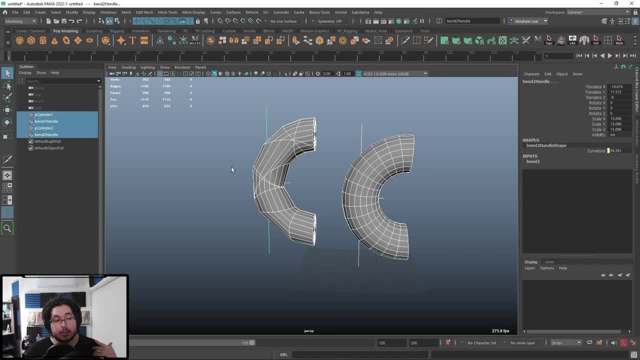 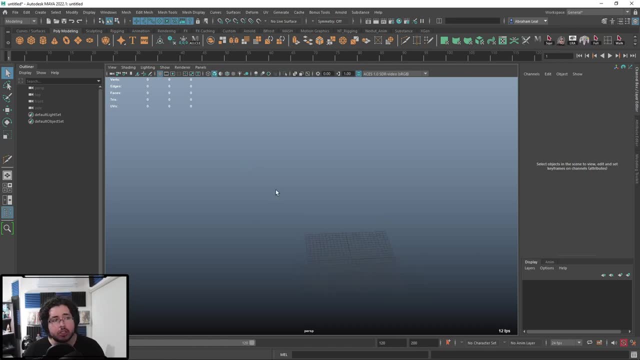 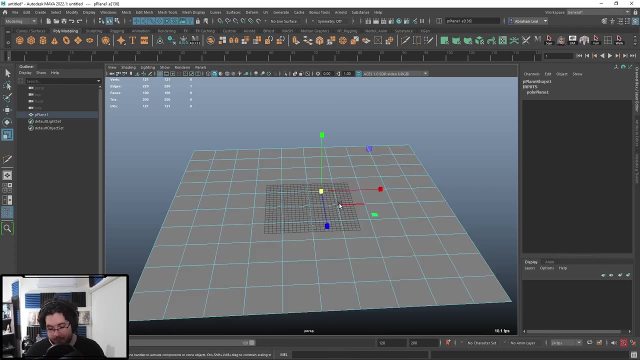 that's one of the first reasons Topology is important and it's necessary to have properly so that deformation works in the best possible way. The second reason to do proper topology is due to something called angles, And usually if you have an object that has a face with more than four sides, like this one right here, which has 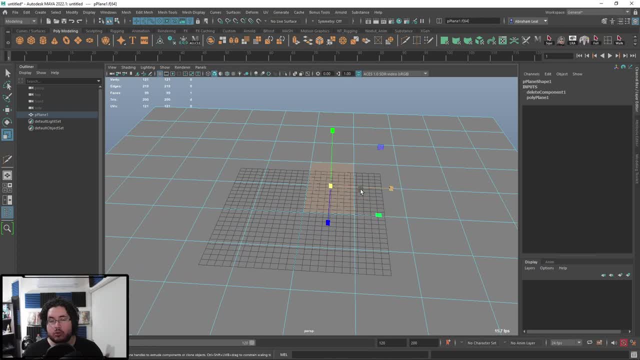 six sides, it's very difficult for softwares to properly do all the math and all the things that they need to do to properly render, modify and deform this sort of shape. So any face with more than four sides we call an angle, And it's very important that we do not have angles on our 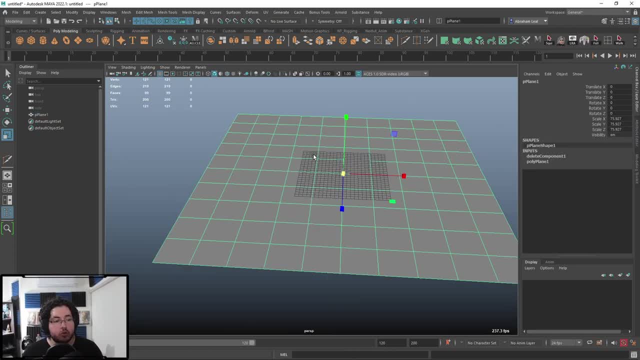 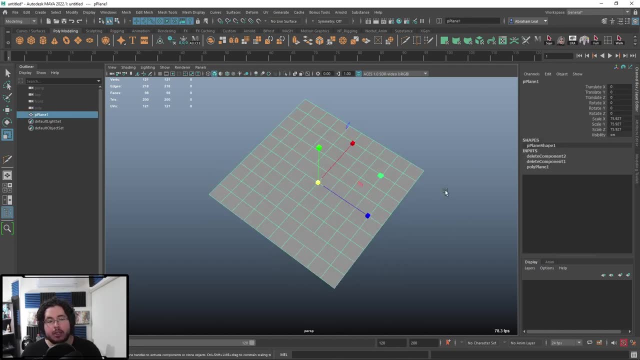 geometry. I'm going to show you a very, very quick little way to to see if your geometry has angles. It's a very nice little trick here inside of Maya. So if you have, like a very complex model and it's like super dense and you're not sure if you have angles or 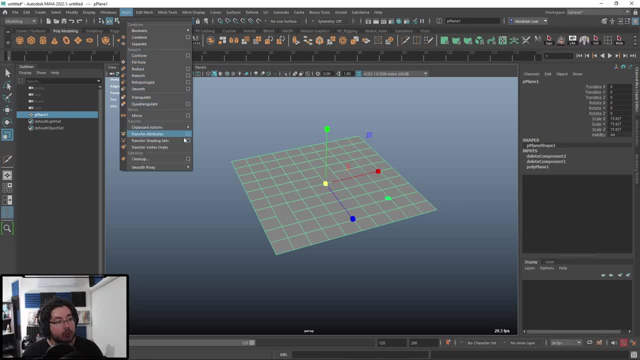 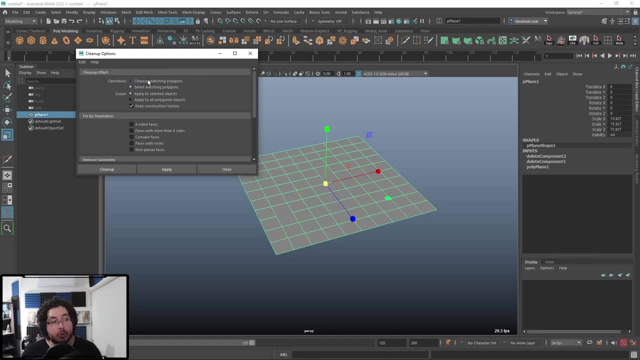 not just click your object and you're going to go into mesh, You're going to go into cleanup And instead of selecting this first option, which says cleanup matching polygons, you're just going to select, you're going to select the second one, which is select matching polygons and which. 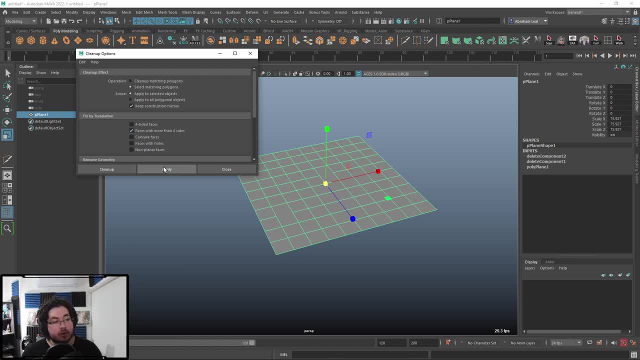 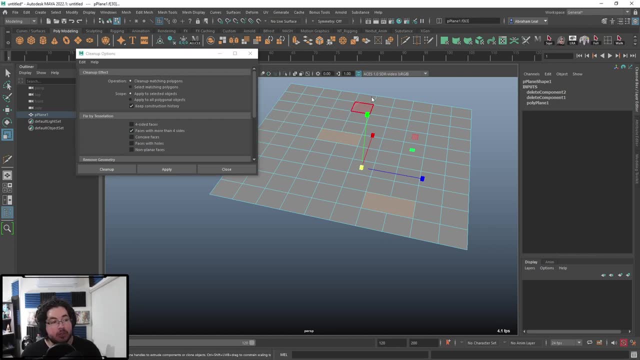 matching polygons we're looking for. We're looking for faces with more than four sides And if I hit apply, it immediately will change my selection to faces and it will hide the faces. So if you highlight the faces that have this sort of effect, if I were to select the cleanup, the only problem 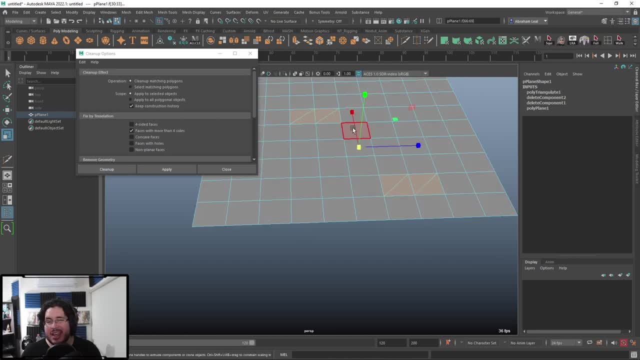 with cleanup is it will do this, It will try to triangulate And, as you can see, it really doesn't work the way we want, right? So that's one of the reasons why, um, uh, we, we don't use this cleanup. 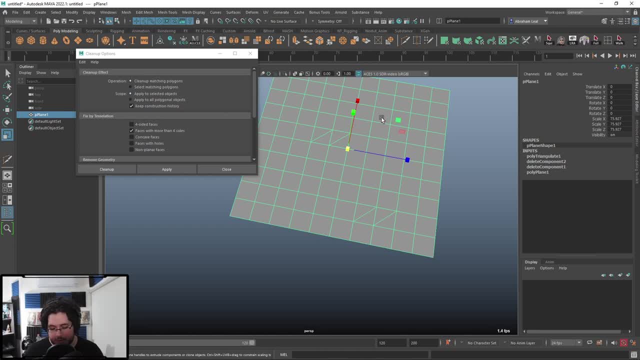 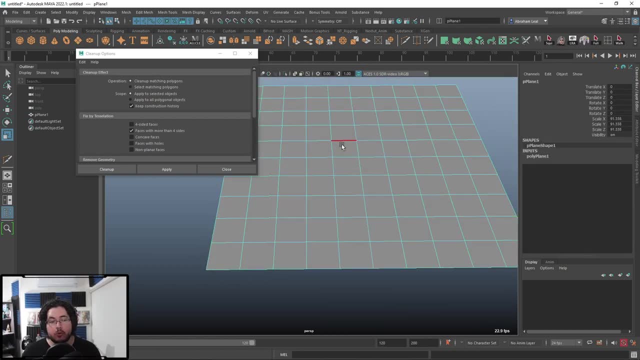 uh, matching polygons, and we'd rather just select them and then manually clean up the things. So another thing that you need to take into consideration is the proportions of your squares. This is a little bit more important for ZBrush and for sculpting than it is for deformation. 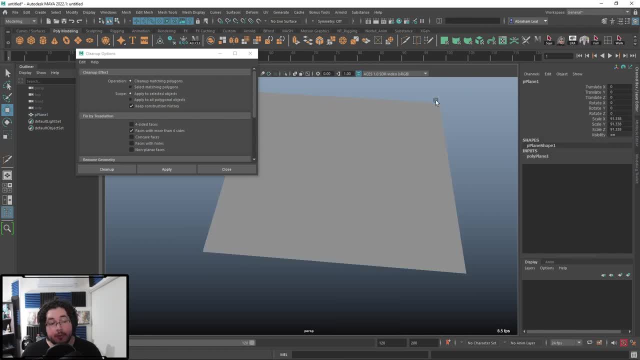 because you can actually get away with, uh, a couple of things. But if you, if you have a mesh like this one right here and you try to bend this compared to like just a regular plane, you're going to see that, even though we have a squares and 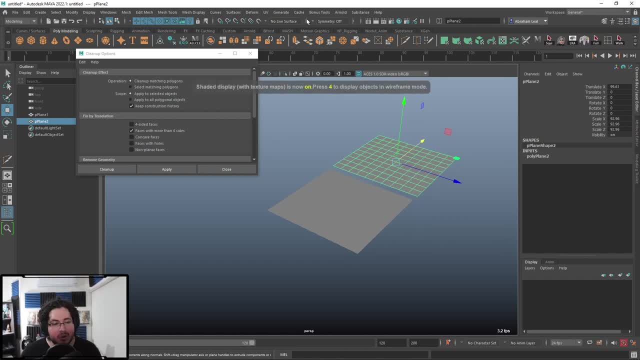 uh and just yeah, just the squares. on both of them the deformation is going to be completely different, And the reason why that's happening is, of course, because the- the way they're distributed is- is different. So if I bend this thing right here, you can see that we can get this very crazy. 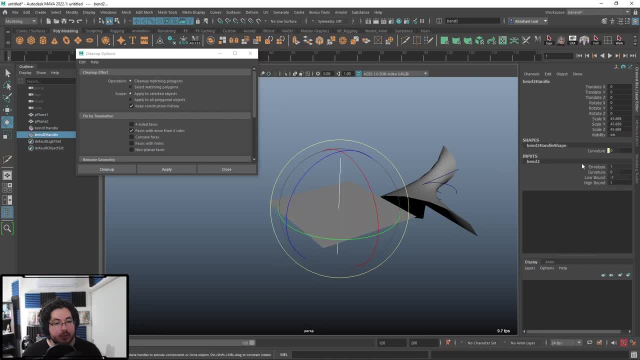 shape. And if we try to do the same thing here with a non-linear bend and just move the curve here and try to do the same sort of twist, you're going to see that we get this sort of error. Why? Because there's not enough geometry here to properly do the twist. Now there might be a case. 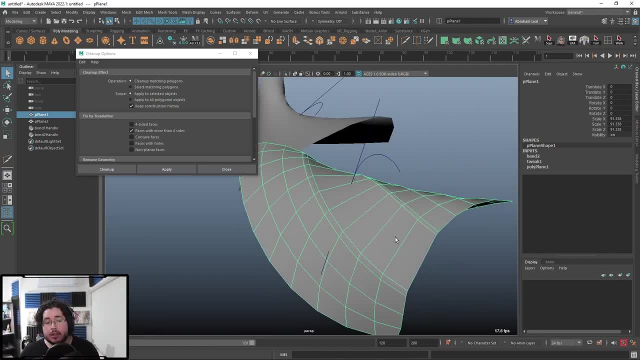 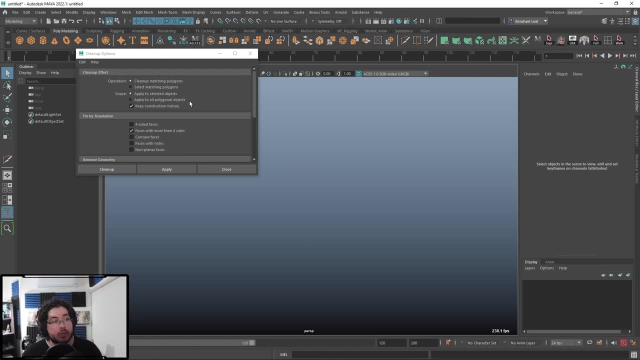 where you need this sort of shape, where you have, like this hard edge in there, That's fine. But usually we try to keep everything like a really, really balanced. Another thing that we try to keep uh clean about topology is the resolution. Like you, usually don't want to work with an object. 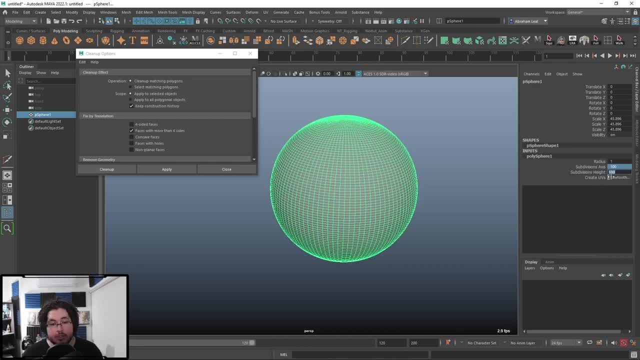 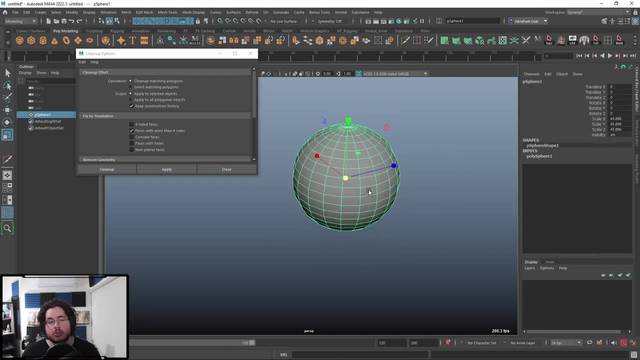 that's super, super high in resolution, Like if we were to go and say: Hey, I want this to be a hundred subdivisions, And the reason why we don't do this is because we have something that was created, I believe, in Pixar. I need to research my history a little bit more, but um, uh at. 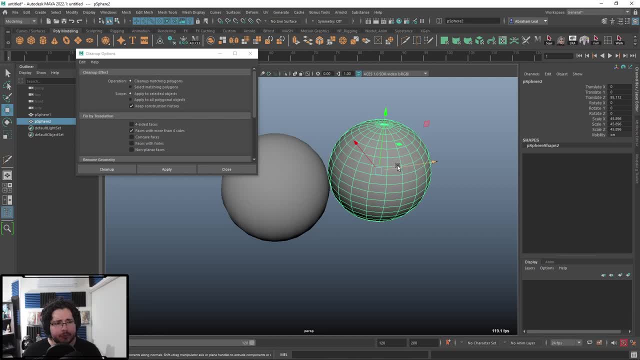 at Catmull, which is one of the founders of Pixar. uh, he developed this sort of technique called the Catmull-Clark. He developed it with a colleague, uh, last name Clark, I believe- And uh, the Catmull. 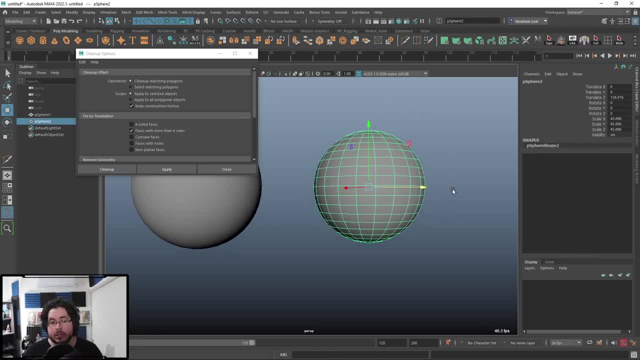 Clark subdivision is when you do this, when you smooth an object and it it calculates mathematically the distance between the edges and the vertices and gives you a smooth surface. And this, uh, Catmull Clark subdivision is present like everywhere. Let me show you real quick. 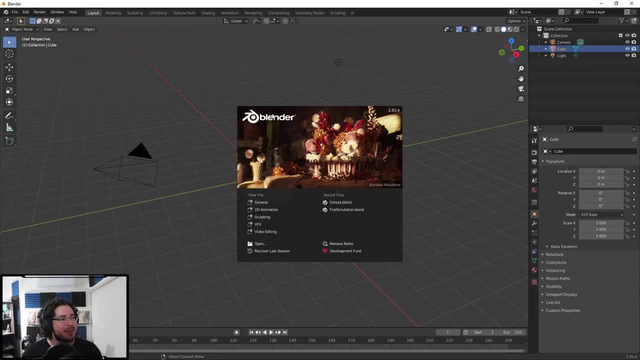 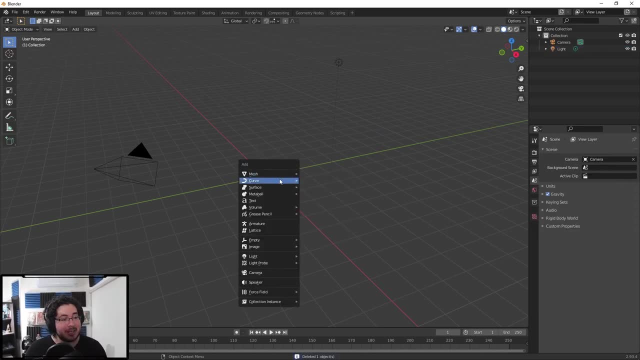 I've been learning Blender, by the way, guys. Uh, maybe if you guys are interested I can do like a quick like my experience with Blender so far it's been. it's been fun, to be honest, Like I've liked doing Blender. So I'm just going to create here a mesh. I'm going to create this UV sphere. 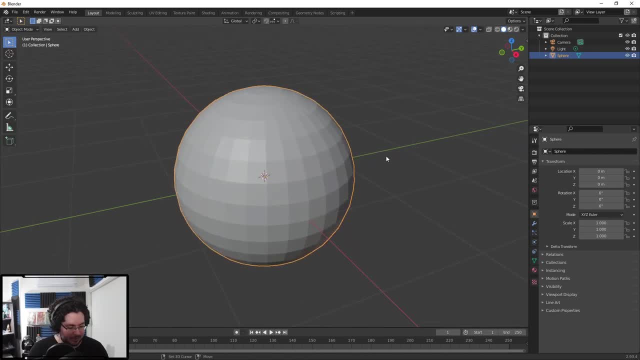 which is like our traditional sphere, And you can see that it's very similar, as in, as in Maya. The only thing I'm still, like always struggling with is the camera, because I'm used to the Maya controls. Um, and in Blender, you guys know that we have these sort of modifiers, which are, uh, things. 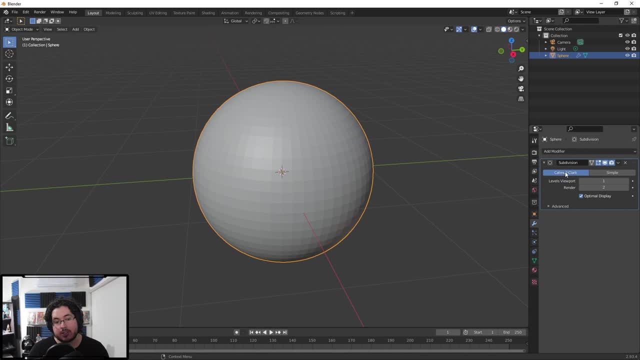 that we use to kind of like come up with things that we need to have in mind. So again we have the uh, the uh. this one is this little uh, this little image here, And we have this thing called the subdivision surface And you can see here that's called Codcit Clark, based again on 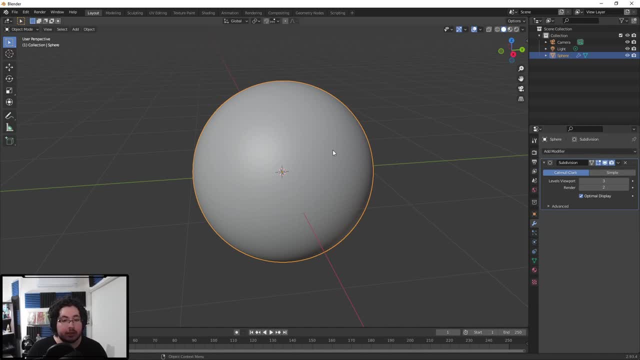 that uh algorithm or or like mathematics that this guy's created so that we can see uh like a smooth surface without actually having the geometry. So this object, even though it it seems like it's super smooth, It's actually not. it's just like this very rough sphere And 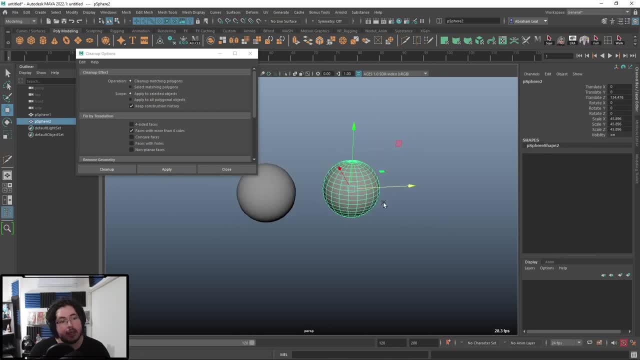 we're just seeing a visualization of how this would look once it's subdivided, like several times. So why topology is really important? because if we're going to be doing subdivisions, we need to make sure that that subdivision is very clean and moves in a very nice way, and i can show you a very simple. 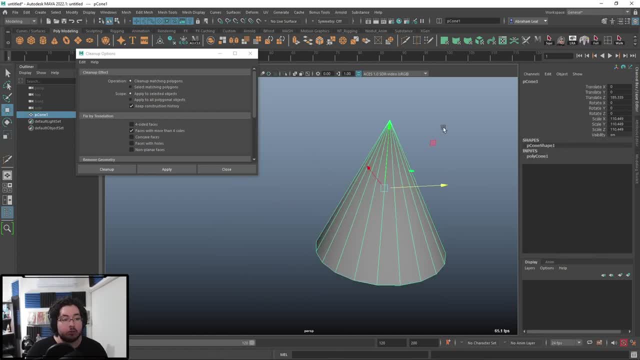 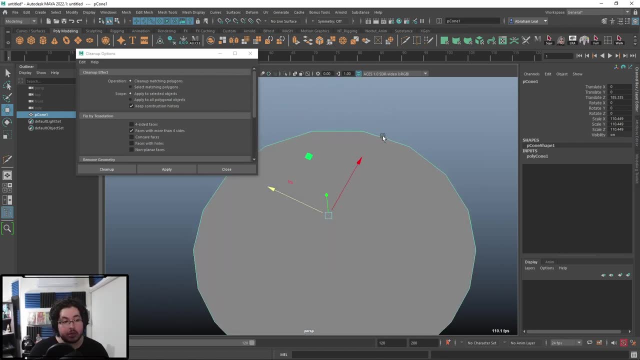 example of how that can break very easily like a cone. you might think: well, this is a basic primitive from maya. why can't we use this cone? well, first of all, we don't have squares, we have a lot of triangles, as you can see here, and second of all, we have a very big angle right here. so if i were 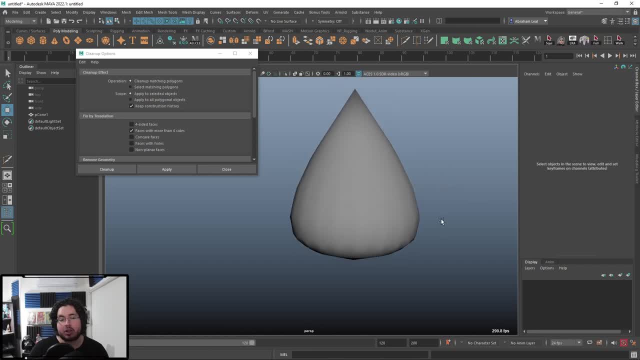 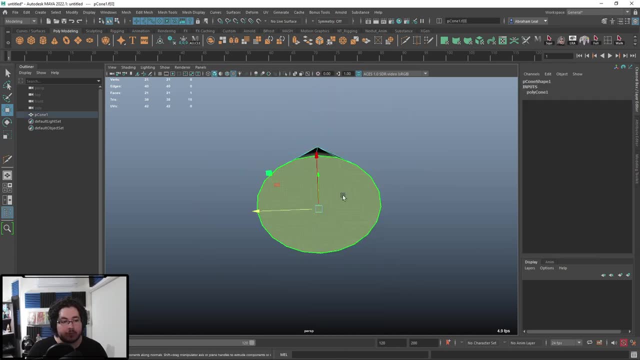 to press number three, you can see that, uh, the catmull clark subdivision is trying to figure out how to like properly do this thing, and and it's not. it's not working. so what would be my answer? well, i would need first of all to convert this into workable topology. so i'm going to go. 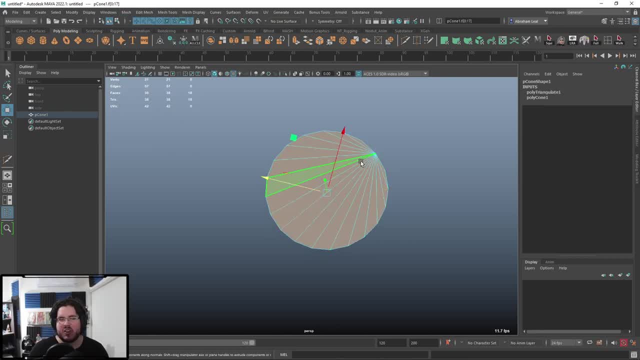 into mesh and hit, triangulate, uh, but that's going to give me like a very bad result, right? i would like to have like something on the very, on the very center. so that's why, where, where i use my poke tool, which is going to create a vertex on the center and then connect every single edge. 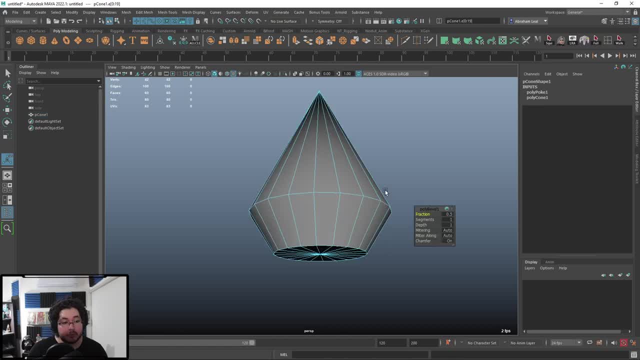 i would then probably like grab all of this edge and give it a bevel, with a small fraction, and like two segments, because we know those bevels are going to hold the bevels, and then we're going to have a bevel, and then we're going to have a bevel, and 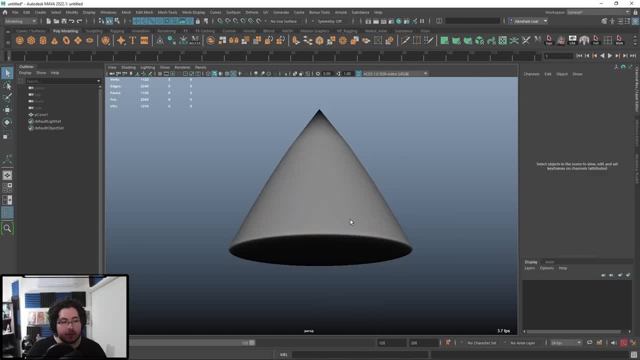 we're going to have a bevel, and then we're going to have a bevel, and then we're going to have a bevel and hold the edge a little bit better. so now you can see that the edge is looking very, very nice. but what about the like, the tip here? what would i do? well, one very cool trick: here we can't do an. 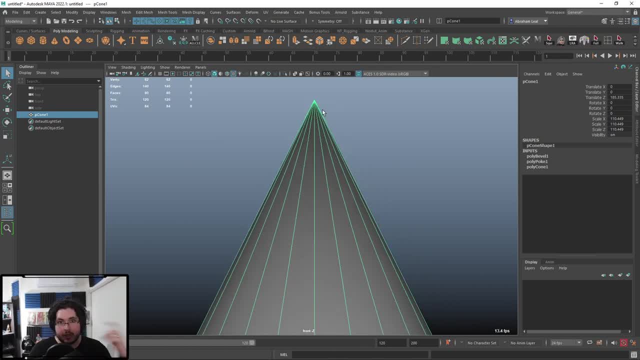 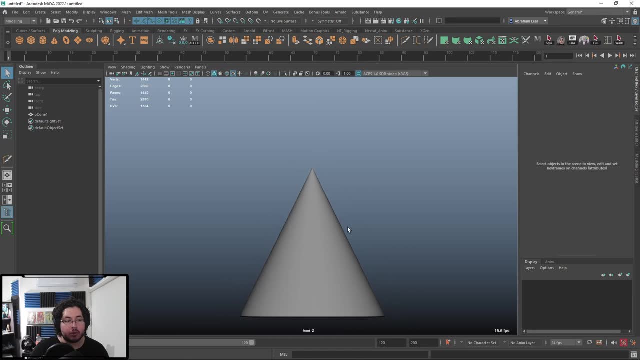 inserted loop because, uh, inserted loops work with with a phase loop, uh with like squares. but we can use a cut tool and just cut really close to the tip right there and that's going to be more than enough to hold the position. so this is a perfectly workable geometry because we have this actual there. 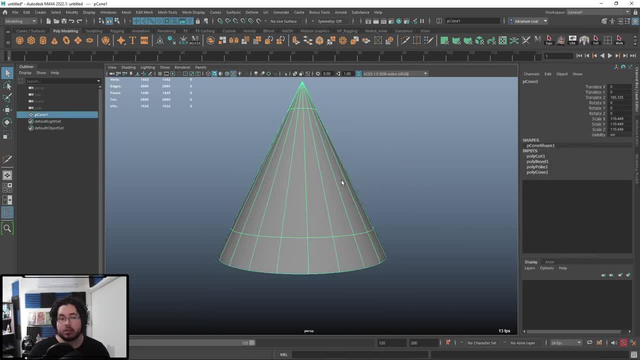 holding the tip and uh, and we get this very nice shape. so that's, uh, the basics of topology. now, uh, i mentioned that i want to show you some very nice tricks. so today's trick- because, remember, these are just short videos, just a quick overview of the things, and tomorrow i'll show you more. 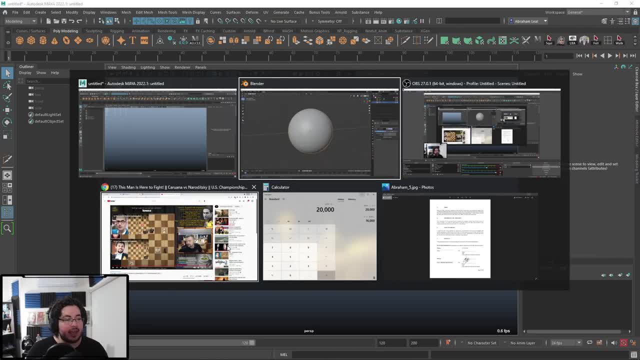 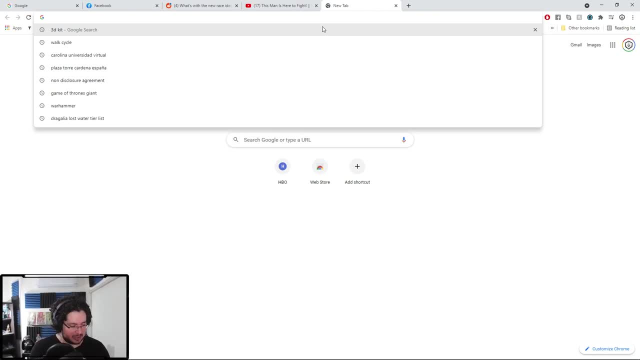 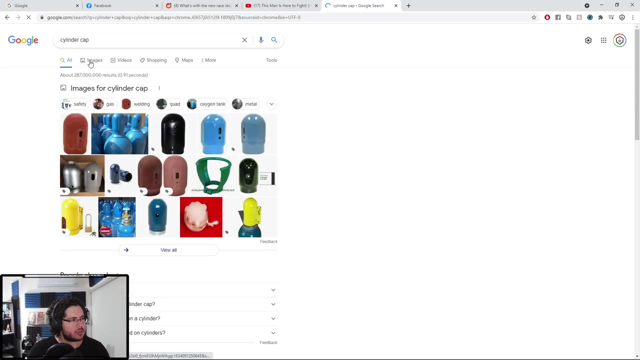 tricks. i'm gonna show you how to do a. um, i was watching my chess videos. i love chess. i've been playing chess for a for like a year now, after, uh, queen's gambit and uh it's very fun. so i'm gonna show you how to do a cylinder cap. you might wonder: well, cylinder caps, just super. 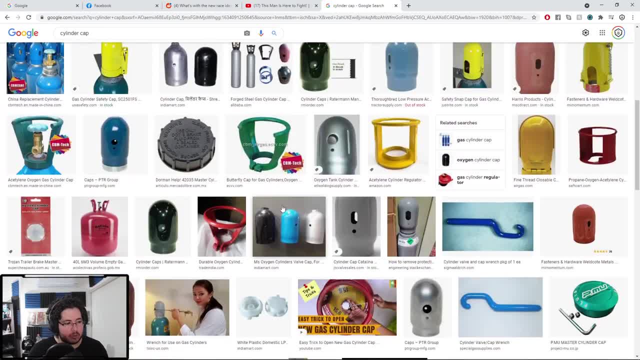 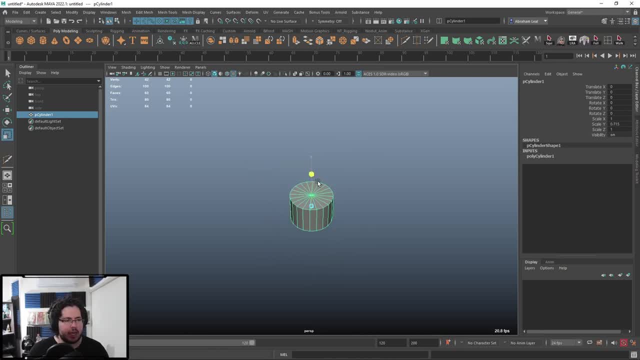 easy, right, like, well, not this one, like, like, just like one for my plastic ball, right, right. and there's a little bit of a problem with topology, especially in game topology. so i want to show you this and the problem is the following. let's say they say: hey, abraham, please, model a. 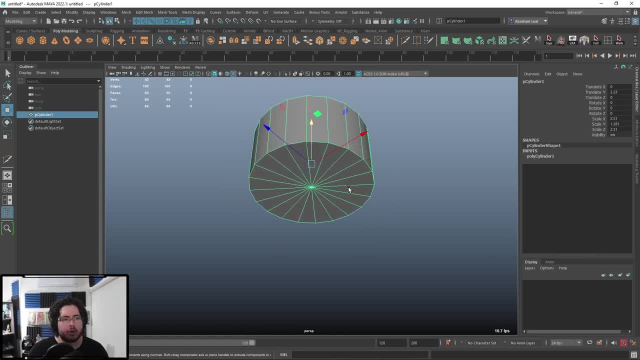 like, just say, a, a coke cap, right, like a like a bottle of soda cap. well, if i just do this, the problem is that the silhouette of the object, as you can see, it's only 20 sides and it's- um, that's very- uh, how would you say- very segmented, right, very fragmented, so so it doesn't look as nice. 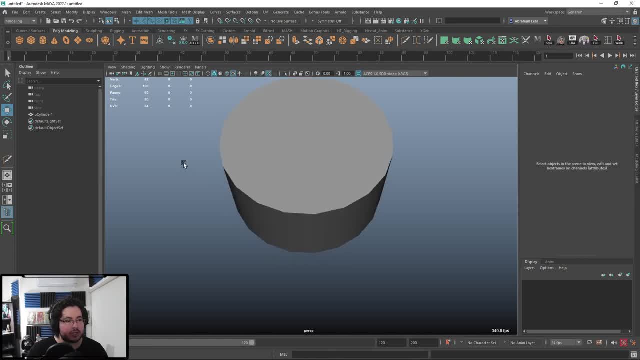 it doesn't look as smooth. you can see like the the corners right there. even if i turn this on, it's gonna, it's gonna try to smooth them, but it's not really working. so some of you might say, well, why not, instead of having a cylinder with 20 sides, let's do 50 sides. 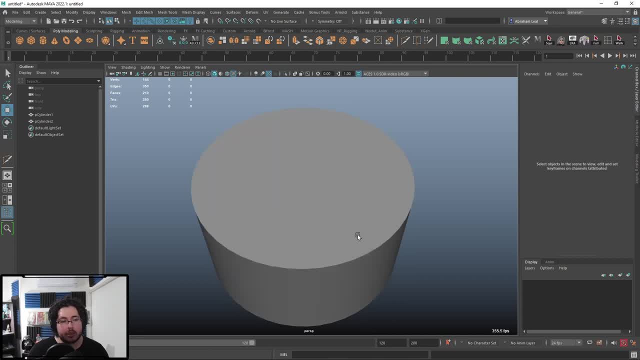 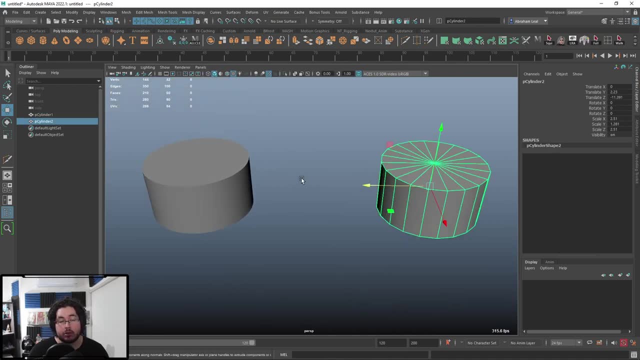 and, yeah, 50 sites is going to give us a super, super smooth cap. it's going to be really, really good. but the topology is also going to shoot all the way up. right now we have 200 triangles, where on this one we only had 80 triangles. so, on game optimization, we need to think about how to. 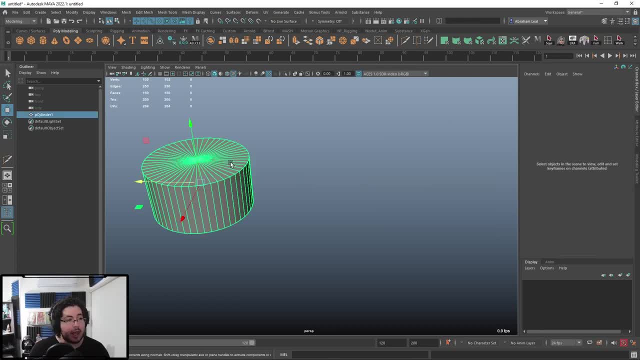 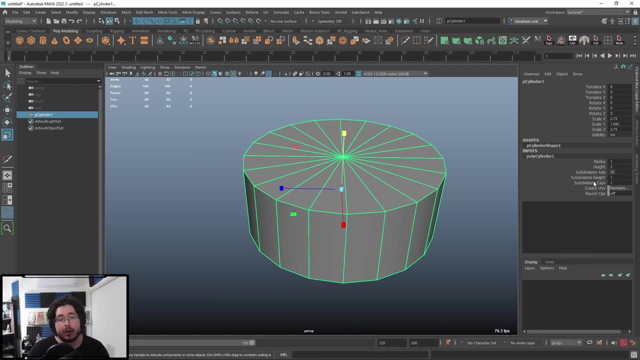 properly optimize this thing. so here's the trick that i'm going to show you. i'm going to grab a cylinder- and this is something that you can do with a lot of things- i'm using a cap as an example, but you can do this with a lot of things- and i'm going to add a 40 subdivisions, which is double. 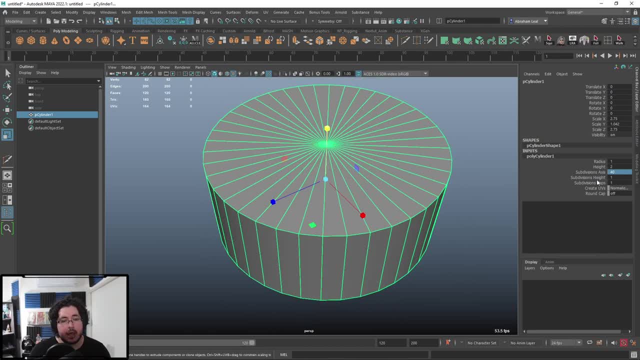 the amount of 20.. so it's going to give me a very round effect, as you can see here. and then on the height subdivisions, i'm actually going to say uh or sorry. on the cap subdivisions, i'm going to say 2, because i want to have a little bit of a border here, this one right here. 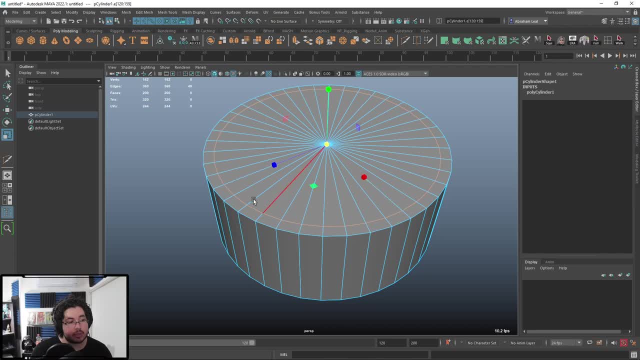 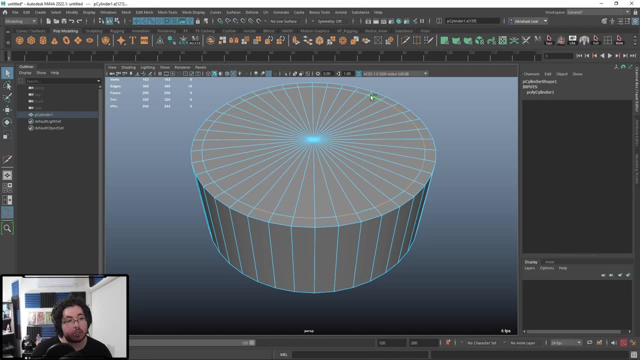 okay, now i'm going to push this guy outwards like this, and then what i'm going to do is i'm going to select one edge loop and then not select the next. i'm going to select one of each. i'm not sure if this or shortcut. there has to be some sort of 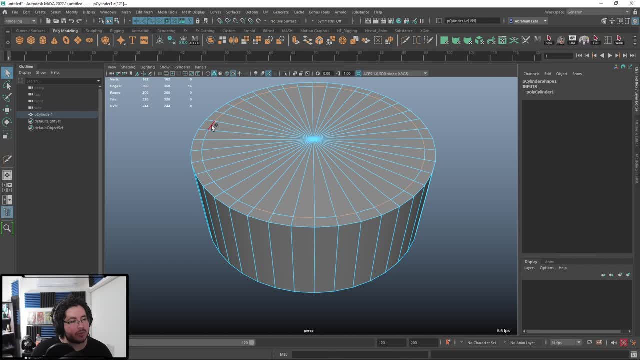 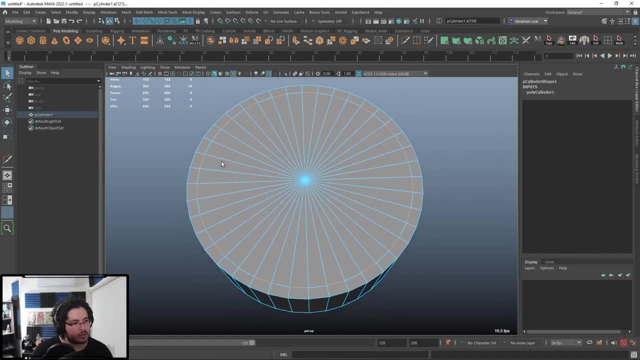 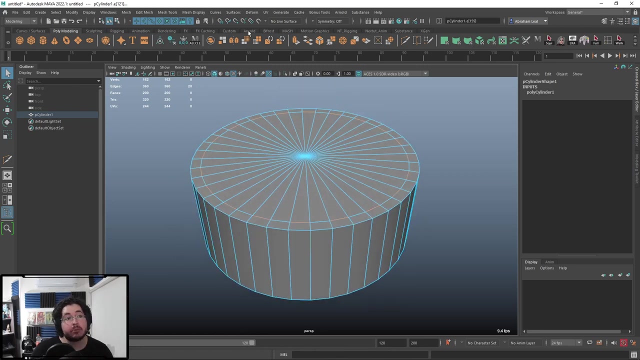 shortcut to to do this in a more like, in a faster way, but this is the one that i know, so i'm just gonna quickly select all of these guys. oh, i messed up somewhere because here, so there, there, there, there and there, and now what i'm gonna do is i'm gonna collapse those edges. so 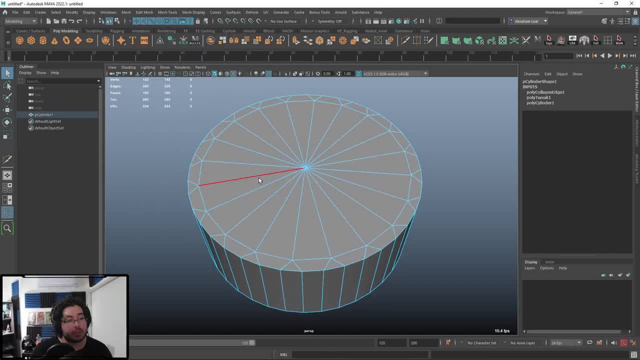 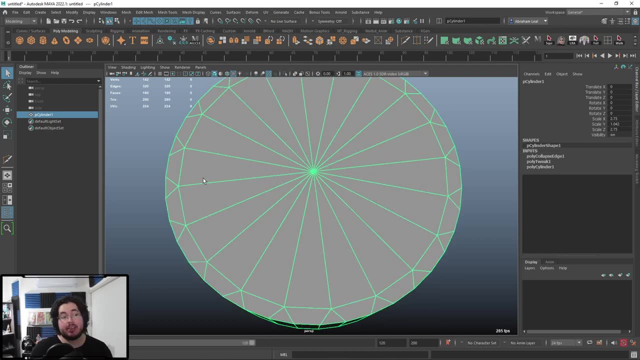 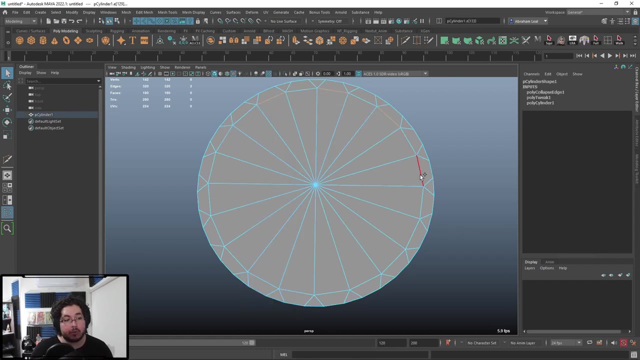 i'm gonna say: edit, mesh collapse, and what's gonna happen is we're actually gonna keep the very round like border on the object, without adding that extra loop here on the inside of our, of our, of our element, and we can even minimize this, uh, more like i can. i could grab these guys right here. 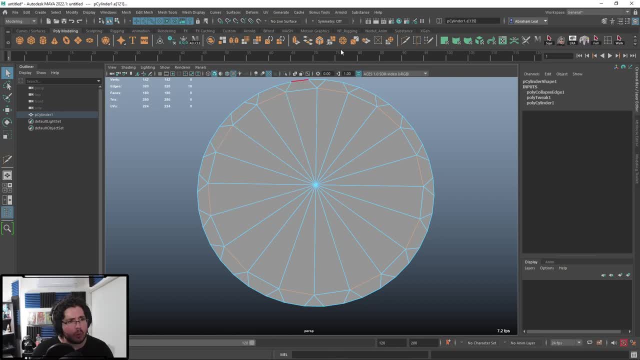 this is something that we do a lot in in game optimization, when the polygons are getting a little bit too big and we want to keep the silhouette, because it's very important for us, because it's going to catch, like that, very nice lighting information. so if i were to collapse, these 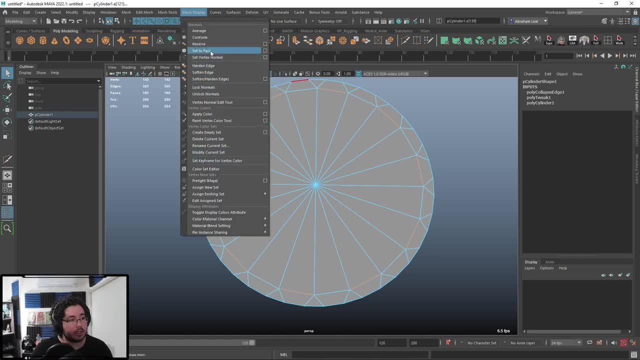 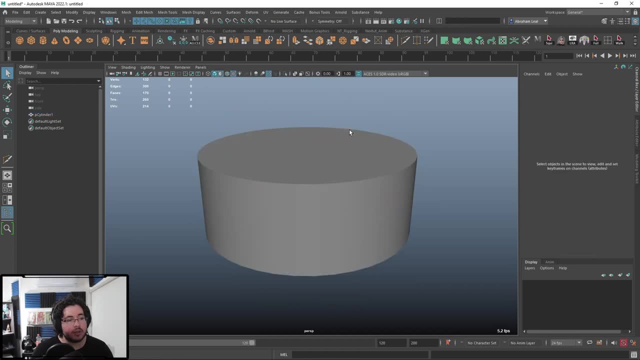 guys as well. where's display? let's go. where is it now? mesh tools? ah, it is mesh collapse. there we go. you can see that now we've created this shape that has a very round edge, but everything's triangle up here and some of you might be wondering: well, is this? 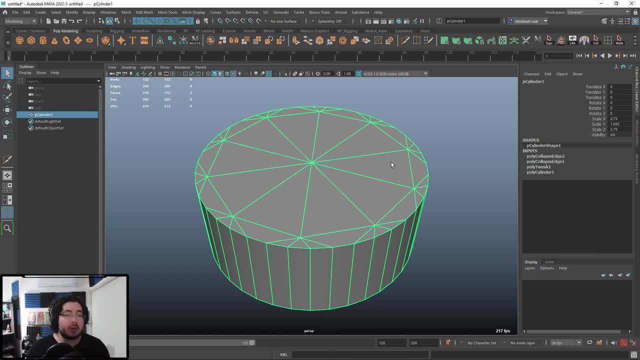 gonna work? is this gonna like? is this functional from a game perspective? it is: as long as this object will not deform. okay, the topology might not look the previous. i would actually leave it like this because i think this looks a little bit better, even though we can save a couple of. 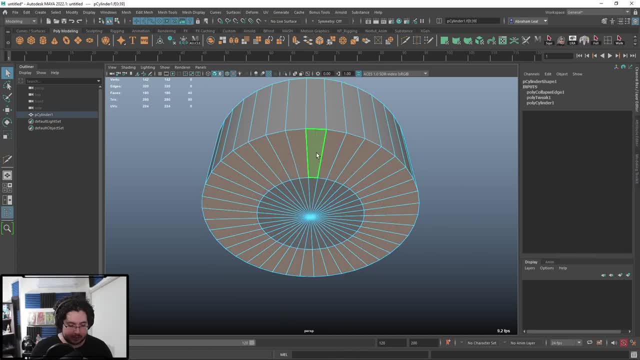 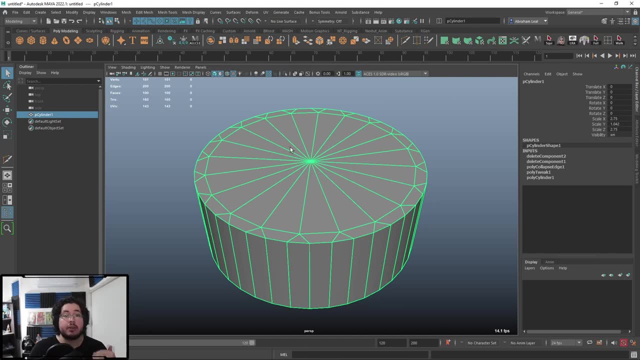 triangles, from minimizing those ones, uh. but let's say, like this guy, we're just gonna have like this cap. so now, instead of having uh 200, we only have 160. so we've uh removed uh 40 edges. but think about like: i've seen things where, where you have like a very, like, a very cool robot. 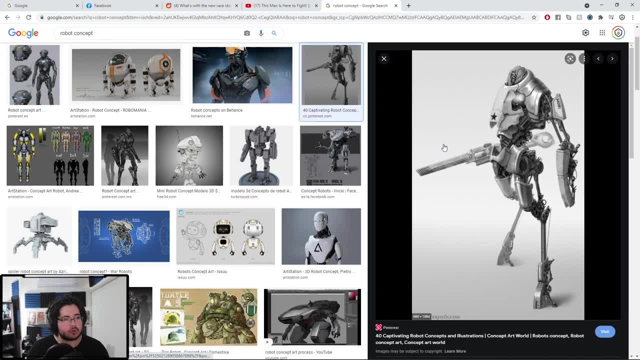 let me look like a concept real quick like. i've seen this kind of things right where there's a lot of uh like circular stuff all the way around. if you were to give all of those guys like the the top resolution that you might need, then the object would be super. 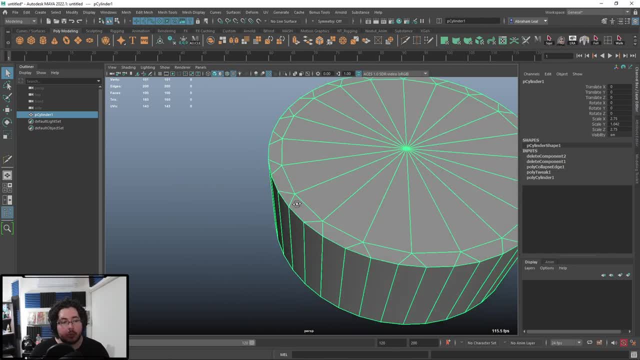 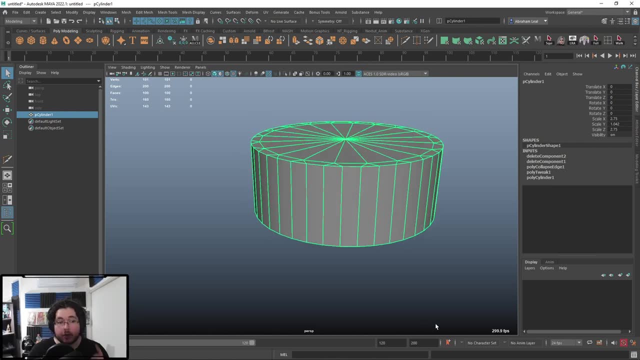 super dense. but if you use this sort of trick where you collapse and leave a couple of triangles helping you hold this silhouette, that's gonna save you some triangles. and this is still a workable geometry for games, not for movies, because if we try to do the edmund clark thing, you can see that 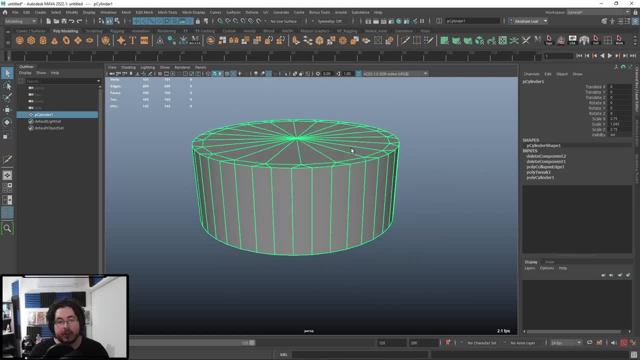 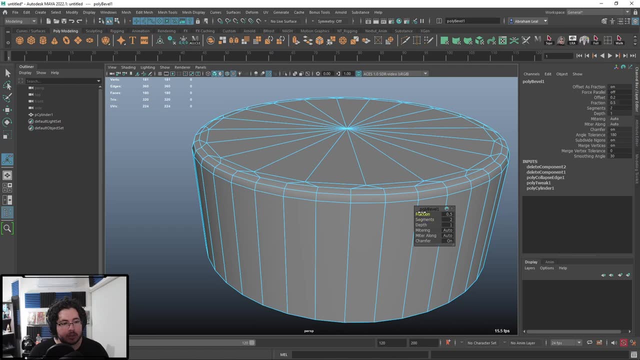 we get this spiky thing, uh, the smooth subdivision, so this would only hold in games. i could, though, if i wanted to give this or give this a little bit more roundness, i could add a bevel with like two segments, and even this would work perfectly for a game, because we're saving some, um some. 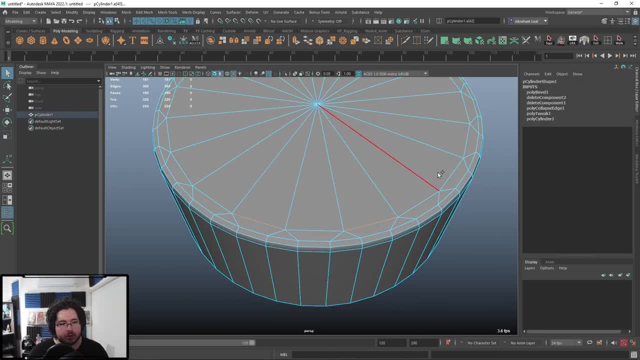 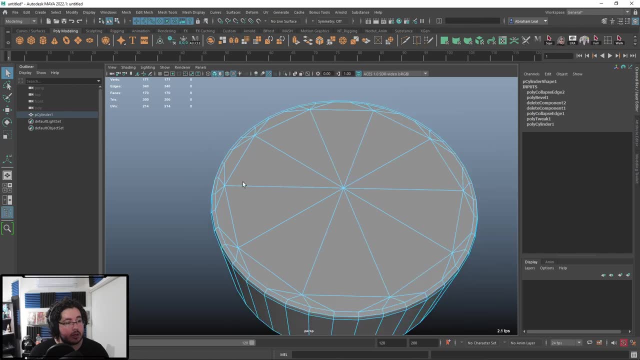 triangles in here. here, though, since we have some more or some extra resolution, i'll probably do the thing that we did before, where i would just collapse this kind of thing. so edit, mesh and collapse, and we'll have this sort of shape, because, at the end of the day, this is just a cap, it's. 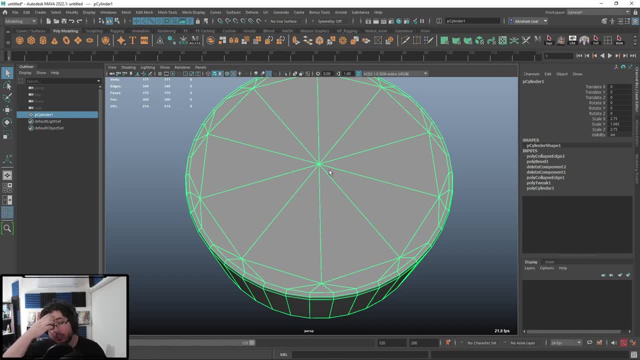 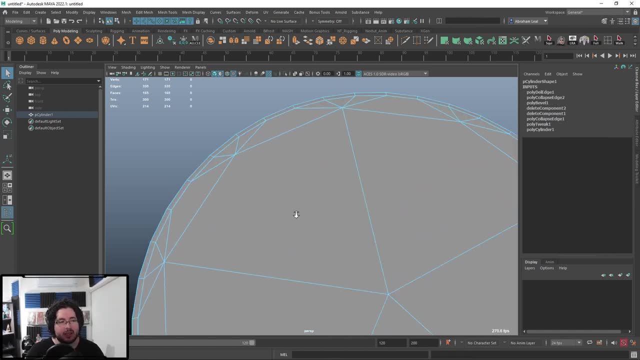 completely flat. so having this sort of topology where everything is a triangle is no big deal. some people might even go all the way to going into this inner guys and just deleting them so that you have squares, but these are like very ugly squares for me. other people would like to. 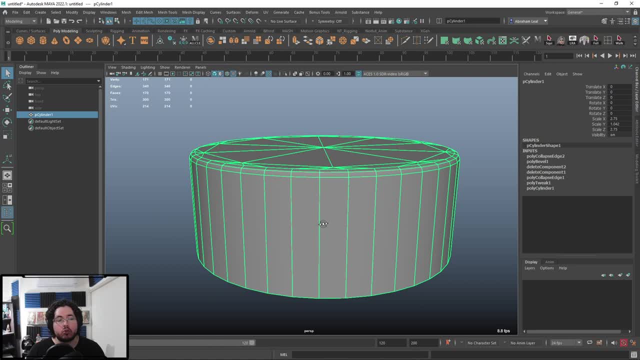 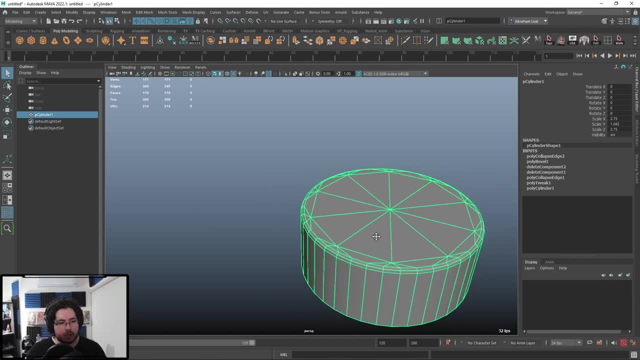 stitch this in a different way. but again, as long as you can reduce the amount of polygons, then you're going to be in a good position. and uh, yeah, that's it for this one, guys. so we took a. uh, we, we saw how to do, uh, this sort of like a simplification. i'm gonna keep one. 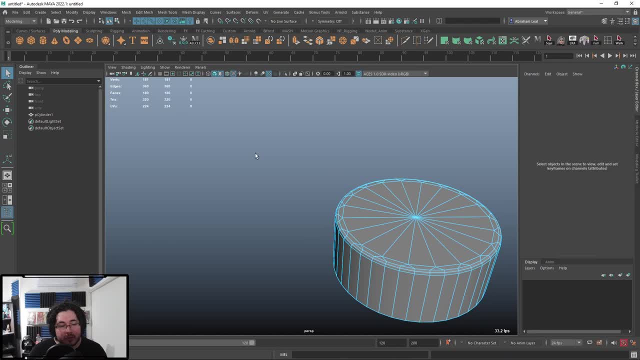 further down here and we saw the bending of the tube and we saw the uh, the importance of um the subdivision, the cadmium clark subdivision. so hopefully with this, especially for all of you guys that are new to 3d and are just learning the basics, hopefully you know or joke and appreciate. 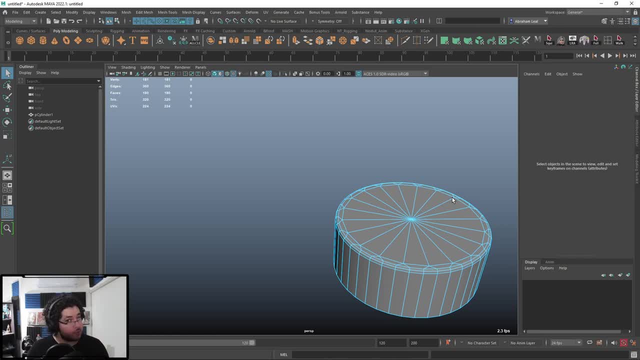 how this thing works. tomorrow we're going to be talking about edge flow and actually is really, really important, so i'm going to be showing you some very nice tricks in in that we can use to modify the edge flow and make sure that our topology in any object that we model. 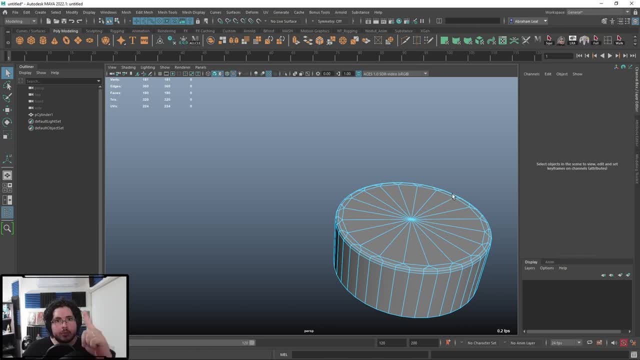 flows in the right way. so hang on tight and i'll see you back tomorrow. wait before i leave, don't leave, don't click out just yet. one final announcement: today's video is the last. or today, wednesday, when this video is up, is the last day to submit your work for the first portfolio review. 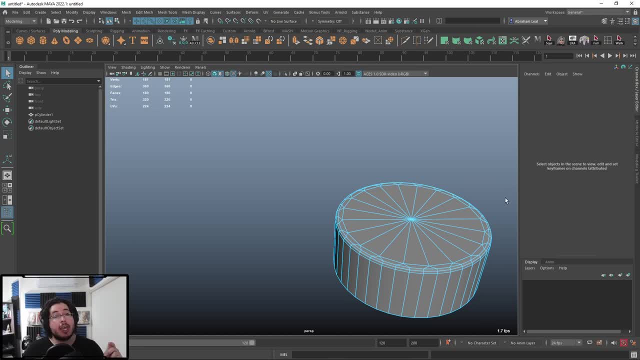 uh, we've been receiving some very nice work, so we're probably going to have a portfolio review weekend. so, uh, saturday and sunday are both going to be videos where we review uh objects for or or from you guys and uh, so make sure to to check the description down here. there's going to be a link. 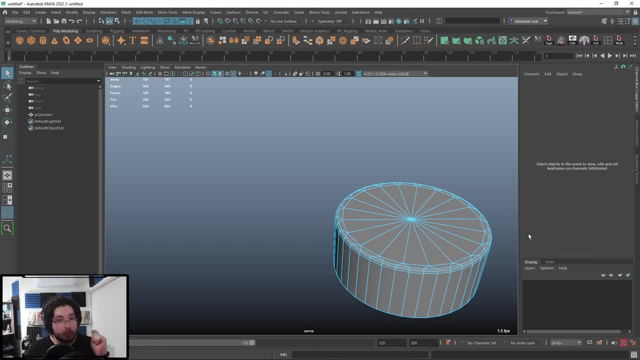 for google drive. create a folder on that shared folder, put your name on it and drop any sort of file that you want me to look at. it could be images, it can be maya files, it can be c brush, c tools, like anything that you want me to check out. uh, we'll check it out during the portfolio. 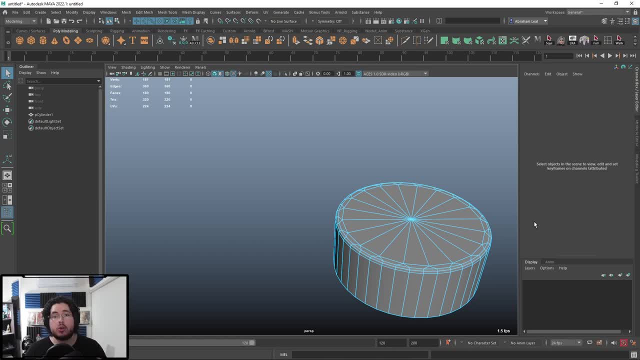 review. i'm going to try to go in order of a submission, so whoever submitted first will get a priority. uh, in case we get like a lot of submissions, but make sure to drop it there. and if you like this content, if you like our videos, know what to do. make sure to like, subscribe, share and now it is true, i'll see you back tomorrow. bye.